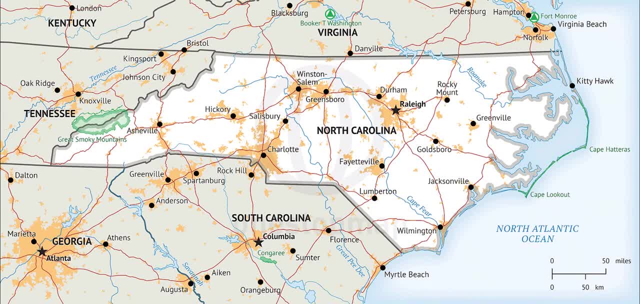 Hello, my friends. This is a map of beautiful North Carolina. North Carolina is bordered by South Carolina on the south, Georgia on the southwest, Tennessee on the west Virginia on the north and the Atlantic Ocean on the east. The United States Census Bureau places North Carolina in the South Atlantic Division of the Southern Region. North Carolina consists of three main geographic regions: The Atlantic Coastal Plain, occupying the eastern portion of the state, the central Piedmont region and the mountain region in the west, which is part of the Appalachian Mountains. 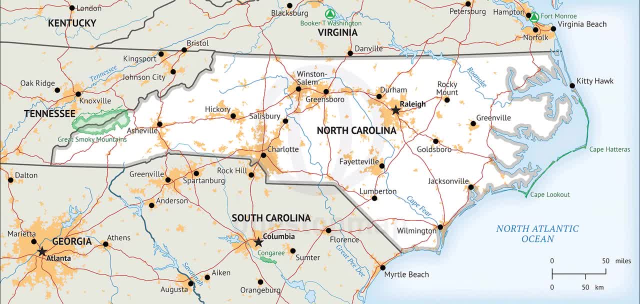 The Coastal Plain consists of more specifically defined areas known as the Outer Banks, A string of sandy, narrow barrier islands separated from the mainland by sounds or inlets, including Albemarle Sound and Pamlico Sound, the native home of the Venus Flytrap, and the Inner Coastal Plain, where longleaf pine trees are native. 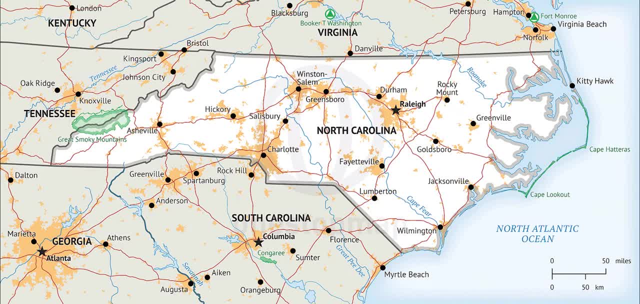 Excuse me, Please comment if you love North Carolina. Continuing. So many ships have been lost off Cape Hatteras that the area is known as the Graveyard of the Atlantic. More than a thousand ships have been lost off Cape Hatteras. 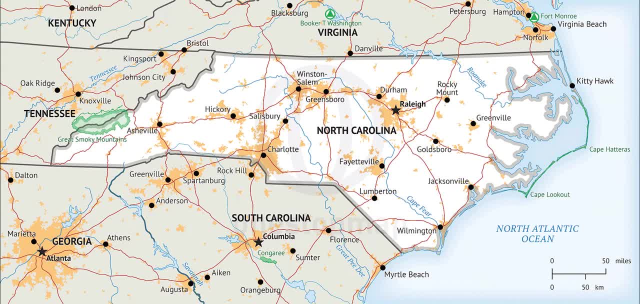 More than a thousand ships have been lost off Cape Hatteras. More than a thousand ships have sunk in these waters since records began in 1526.. The most famous of these is the Queen Anne's Revenge flagship of the pirate Blackbeard, which went aground in Beaufort Inlet in 1718. 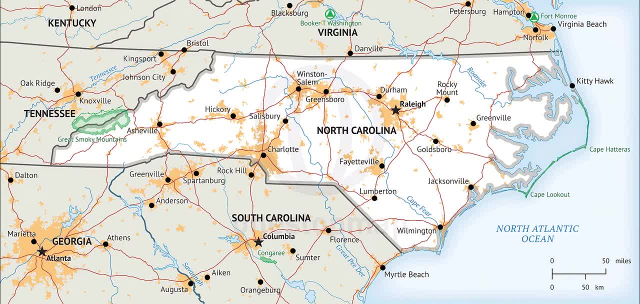 The Coastal Plain transitions to the Piedmont region along the Atlantic seaboard fall line, the elevation at which waterfalls first appear on streams and rivers. The Piedmont region of central North Carolina is the state of North Carolina. The Piedmont region of central North Carolina is the state's most populous region, containing the six largest cities in the state by population. 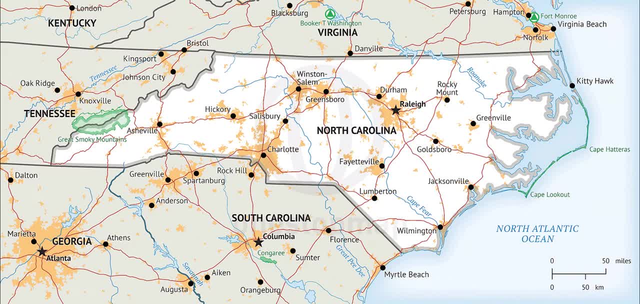 It consists of gently rolling countryside, frequently broken by hills or low mountain ridges. Small, isolated and deeply eroded mountain ranges and peaks are located in the Piedmont, Including the Sorretown Mountains, Pilot Mountain, the Uari Mountains, Crowder's Mountain, King's Pinnacle, the Brushy Mountains and the South Mountains.